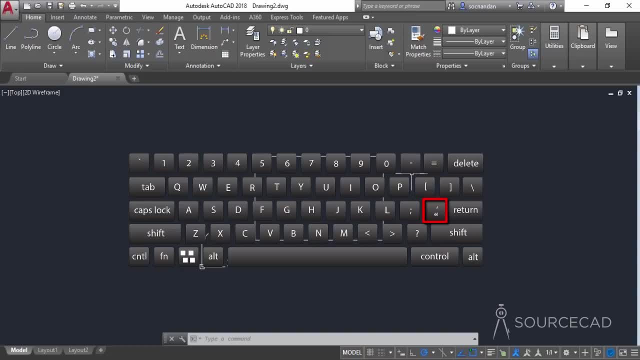 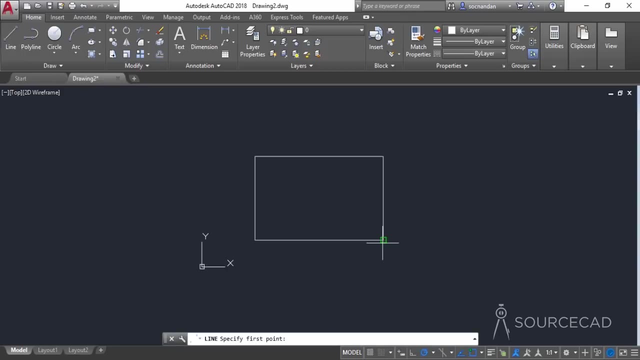 feet. sign on your keyboard And here's the key which should be selected. And for selecting the inches, you need to select the same key by pressing and holding the shift key. Now let's go to the line tool, And this time I'll start with this point, but I'll not click on this point. Instead, I'll 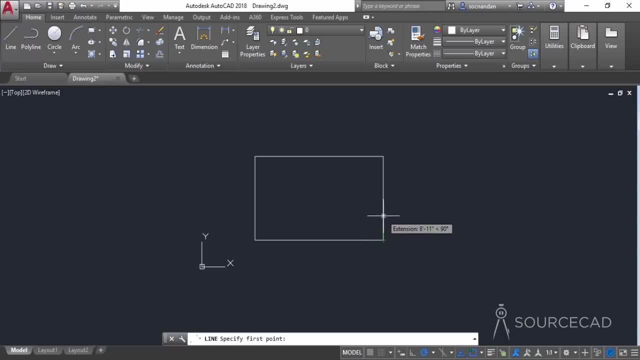 simply track it in upward direction. And when I track it in upward direction, you'll see this extension option on this tool tip And if you're not able to see this option, this object snap. click here and select this extension option. Now I'll click back here. 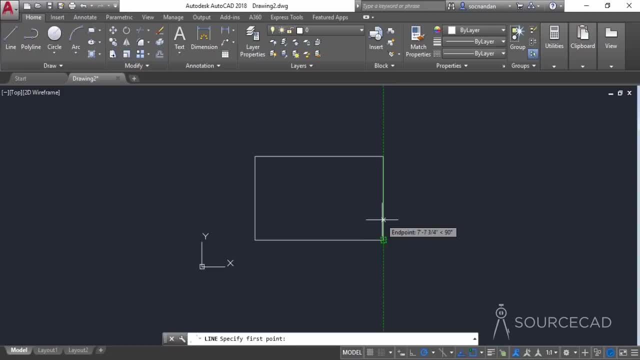 Once again, I'll go to this point and track it upwards and enter a distance of 15 feet and press enter. Now move it in this direction. enter a distance of 12 feet, press enter and move it downwards like this. Now press enter again to repeat the line tool. Click on this point. 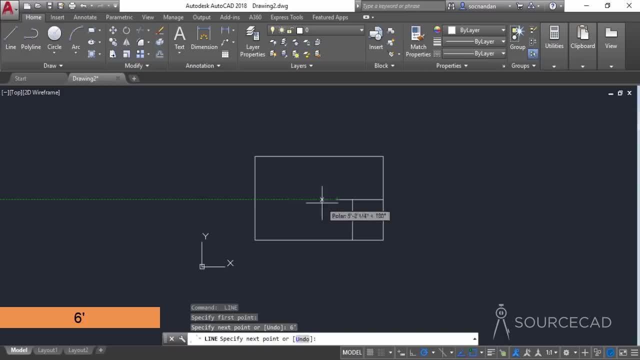 and enter a distance of six feet, press enter Now. move it in this direction. enter a distance of 10 feet, press enter Now. join it with this point. Make sure that it is connecting this line at the intersection point and not this midpoint. So here we need to ensure that it is connected at. 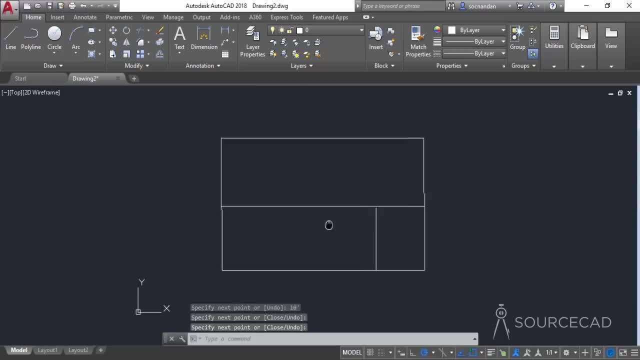 this intersection point like this: All right, so here we have it. Now go to the line tool again and go to this end point and join it with this one. this intersection point: Press enter again. select the next end point. join it here. Now the boundaries of this floor plan is complete. 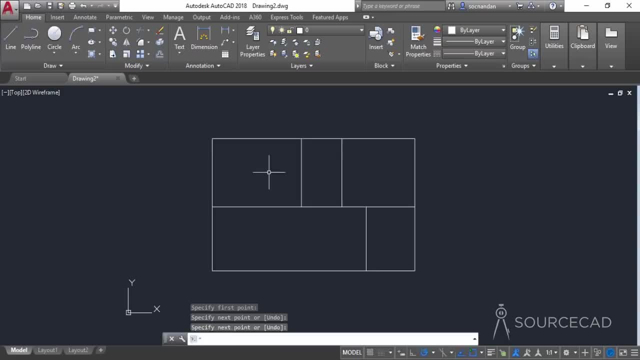 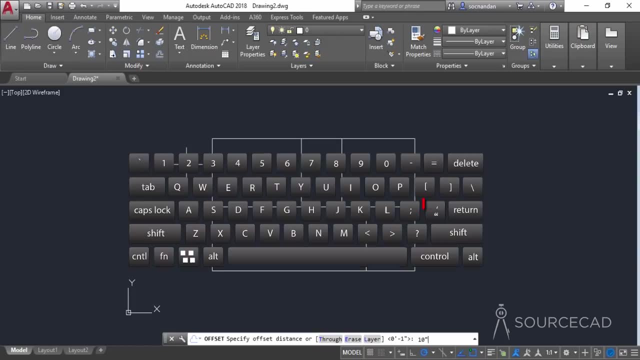 We need to add thickness to the wall. For that I'll go to this offset tool and enter the offset distance of 10 inches. And for inches, you need to select this keyboard key and you need to select it by pressing and holding the shift key. Now press enter. 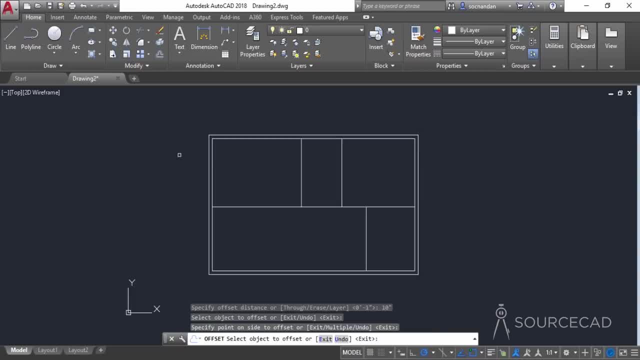 and click on this rectangle and click outside. Now press enter again and press enter again to repeat the offset tool. Now, this time I'll select an offset distance of six inches and press enter. Now click on this line. offset it in upward direction. upward direction, upward direction. 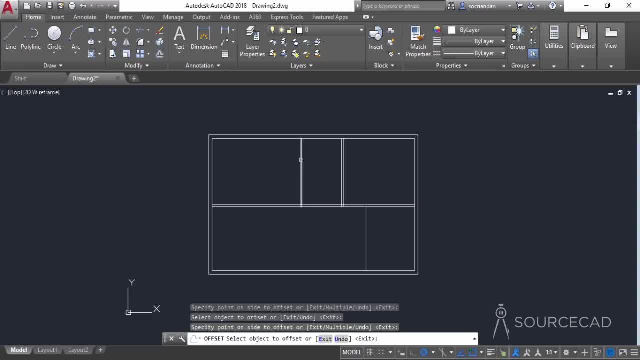 and this one also Here. move it towards right and move it towards left. Move this line towards right. All right, now we need to add one more line over here, and for that I'll once again select offset and add an offset distance of 10 feet and press enter. 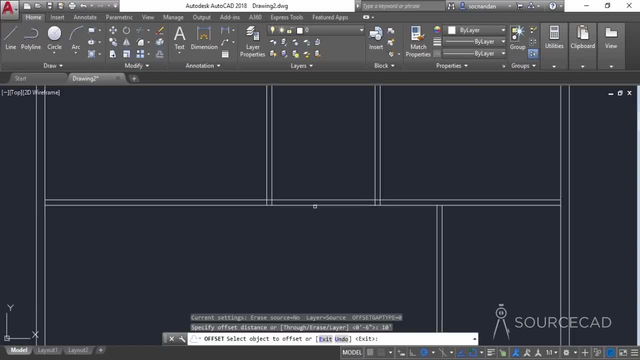 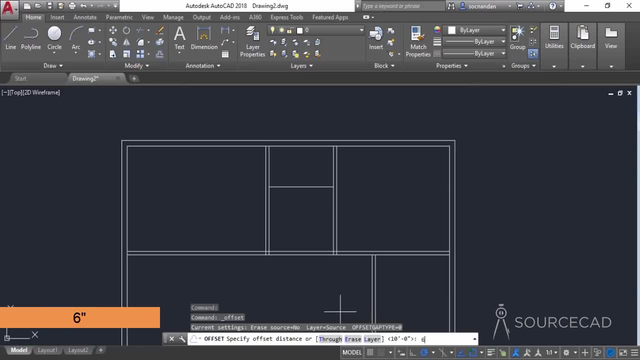 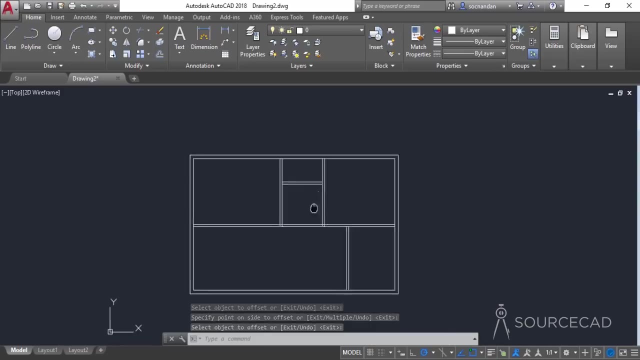 Now click on this line, this one which is on the bottom, and click upwards and go to offset and select an offset distance of six inches, press enter and move it upwards. All right, now we need to clean this geometry a little bit, and for that 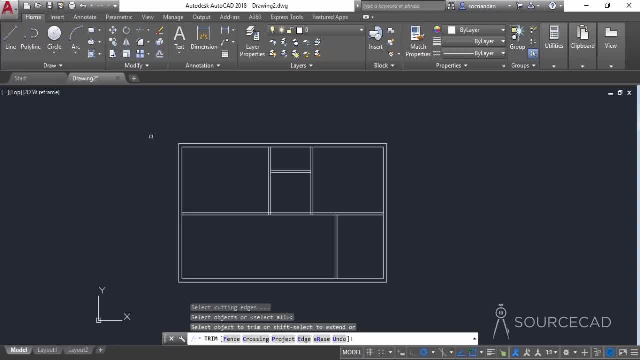 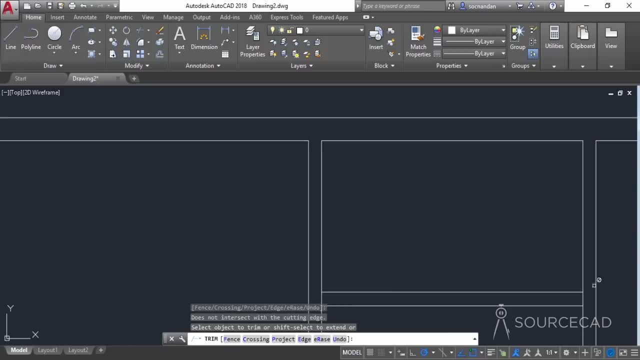 I'll select trim tool, So select it and press enter. Now carefully remove these parts of the drawing. So this area should be cleaned, and here also, here also, here also. So, wherever these lines are intersecting, simply clean them. 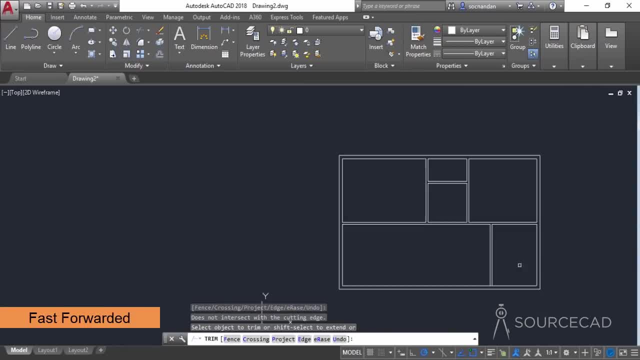 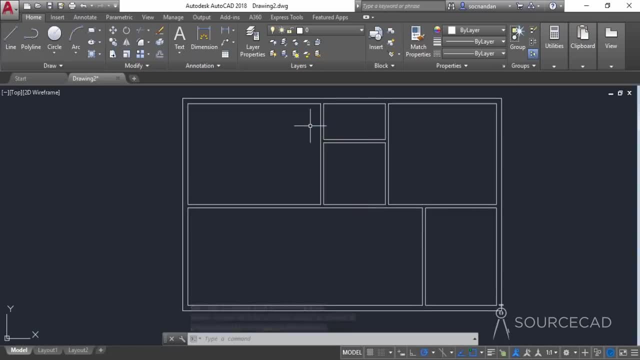 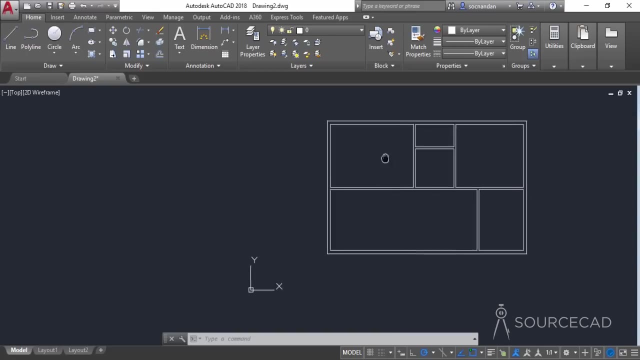 all right, the drawing is now complete. now we'll start by adding two different blocks and we'll start with the door and window, and before that we need to make the door and window. so we'll make our own door and window here. but before making those blocks i'll go to this layer: properties. 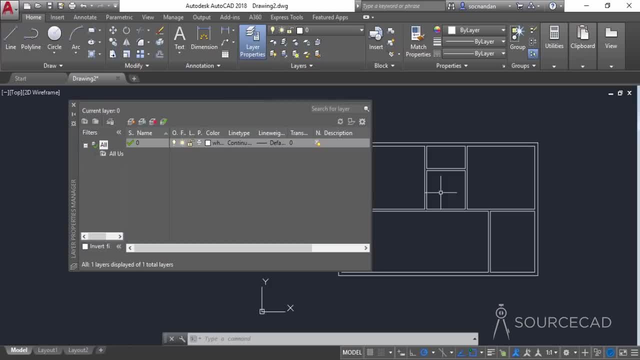 now click on this layer properties and add some layers to the drawing. so we need to add these layers because we will place different objects on different layer for easy classification, and that's the general way of making these drawings, and you should also try to put different kind of 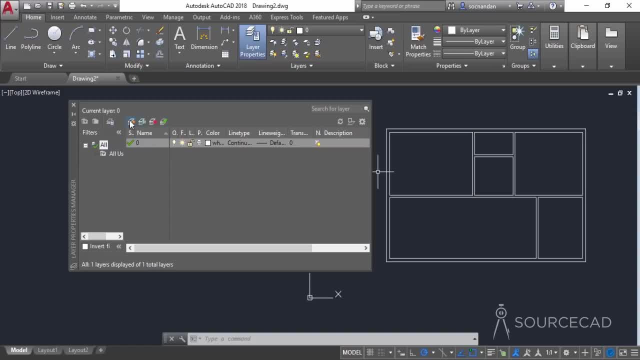 objects on different layers. so i'll click on this new layer option and i'll add a new layer door. click on this again and type window the same icon and type blocks, hatches, text, dimensions. and that's it for now. so i'll add different colors also, so i'll go to this. 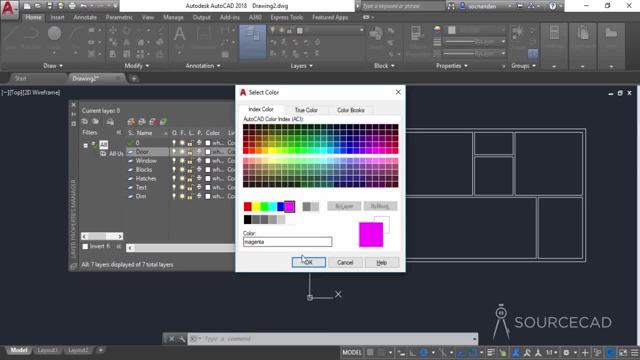 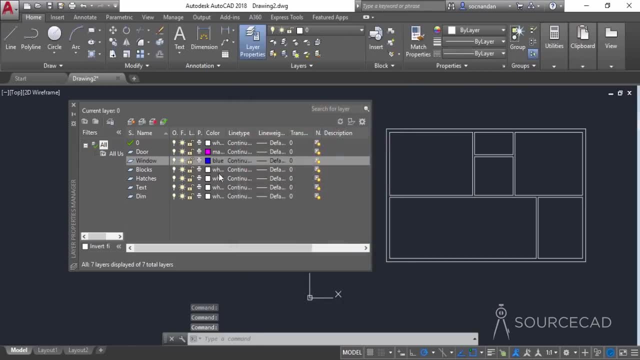 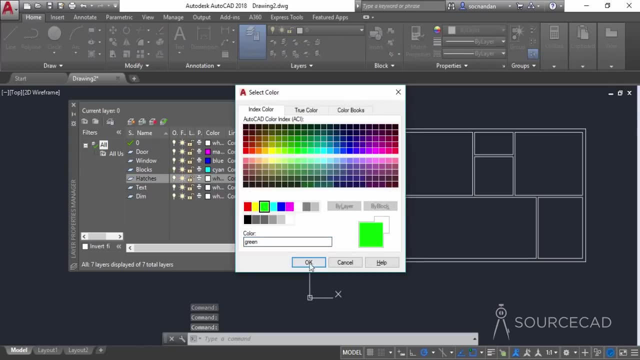 door and i'll add this magenta color to door. i'll go to window. let's add this blue color and let's go to blocks. add this cyan. for hatches, i'll select green, for text let's select yellow, and for dimensions, i'll select this pink color. all right, so we have added colors and these colors. 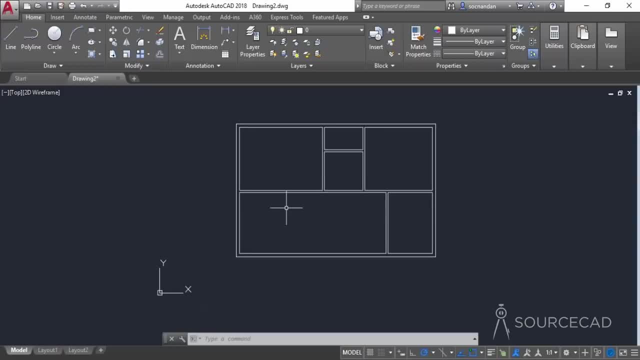 will be used to differentiate between different objects of the drawing. so now we can start with the door block. so go to this drop down, change it to inside of the door block. and now we can start with the door block. so go to this drop down, change it to inside and go to the door box and then go to 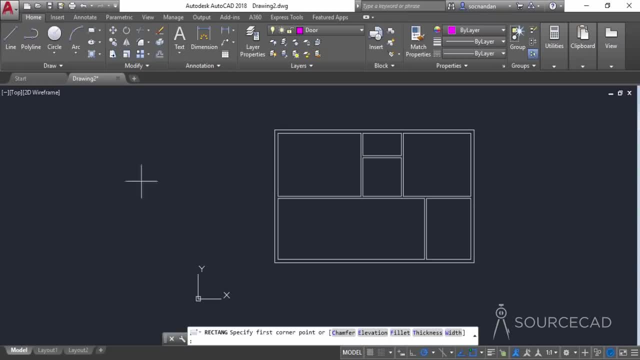 to door and now click on this rectangle tool. click anywhere in the drawing area and type at: and the length of this rectangle should be three inches and the height should be three fit and press enter. so all right, here we have it. now make another rectangle, a small one, and this time i'll 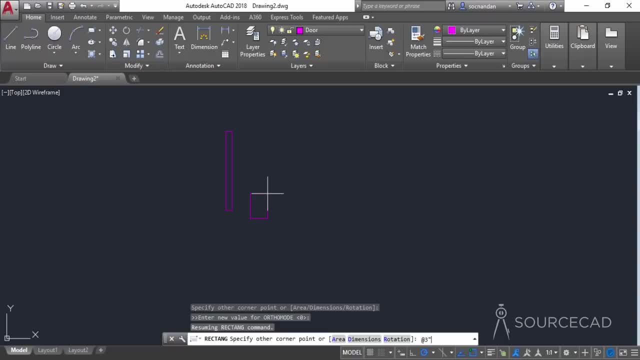 type at a length of three inches and a height of six inches, and press enter. all right. so here we have it now simply move it on this end point here, just like this. now i'll go to this arc tool and select this center start, end. now click on this point. that will be the center point. 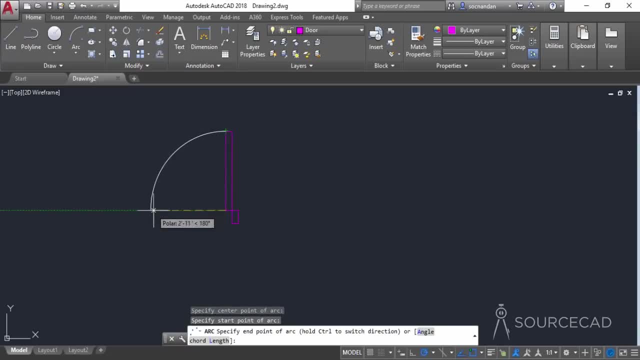 the start point and the end point along this x axis. now make a Werehead copy of this small rectangle and simply move it on this endpoint like this. So our door block is ready. Now we only need to make a variation of this door block, and for that I'll make a copy of. 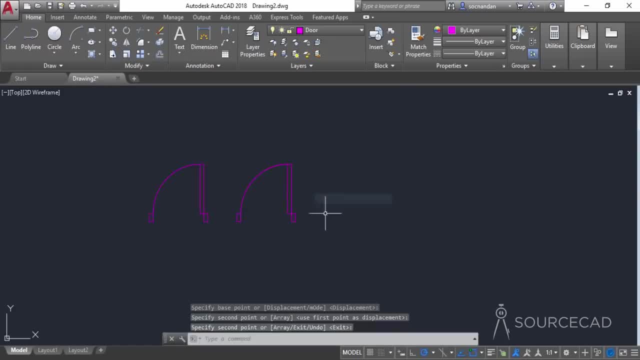 this. So select copy tool. and here we have it. So that's the original one and I'll just make another copy here. and for making the next copy, I'll select this mirror tool, Select mirror, select it all and press enter. Now click on this point. and click on this point and press. 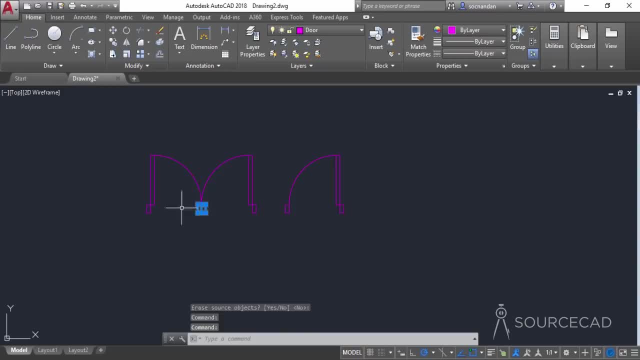 enter. Now we need to remove these two rectangles. These rectangles are no longer needed and here we have it. So we have these two variations of the door block. Now let's make windows, and for windows I'll once again select rectangle. and before doing that, 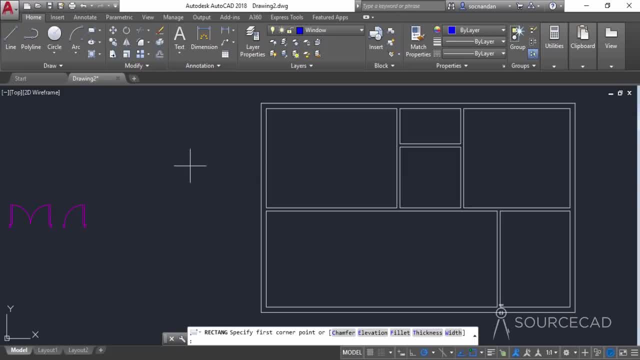 let's change the layer. So I'll change the layer to window. All right, now click anywhere in the drawing area. Let's type at- and the length is five feet, comma, the height is six inches and press enter. So as you can see that, due to the dark color of this window, we are not able to see it, 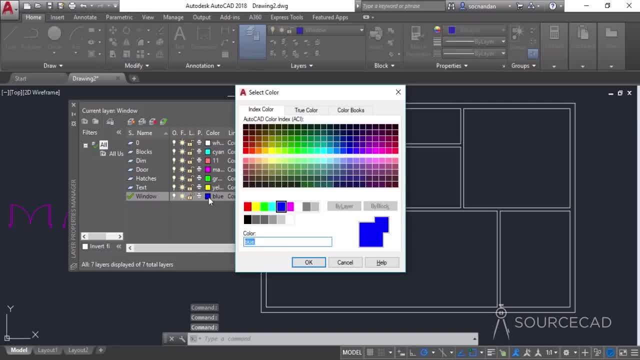 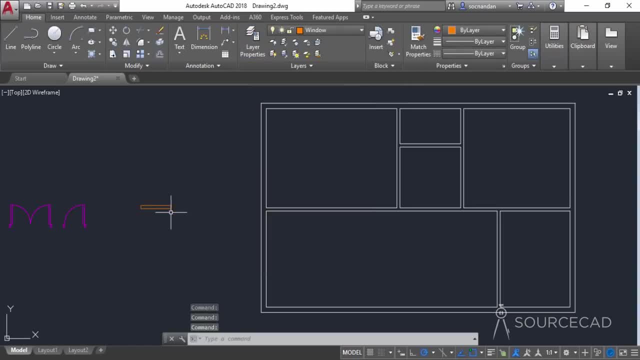 quite properly. So I'll change the color of this window to five feet and press enter, So, as you can, the color of this window. So I'll click on this box and change it to this orange color and click on okay, Close it. So there we have it. Now it's quite clearly visible. All right, now let's explode. 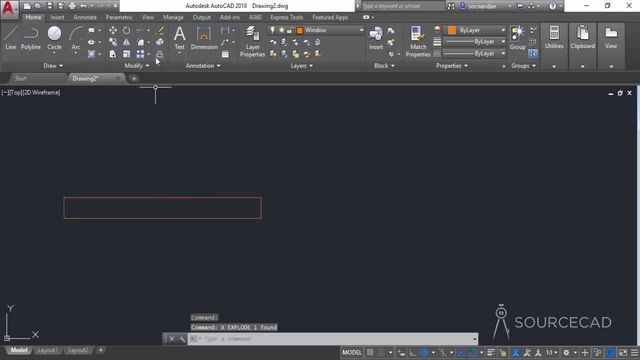 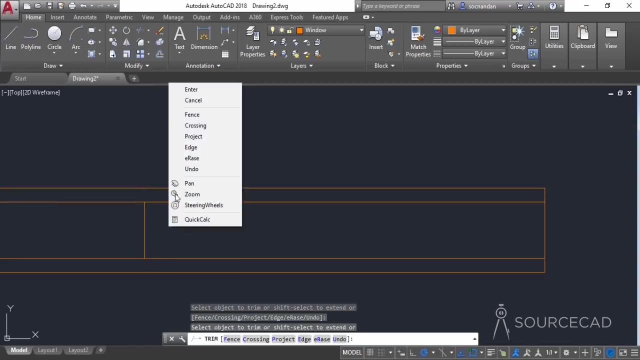 this drawing and click on offset. Enter an offset distance of one inch. Offset it downwards, Offset it here. Now make a copy of this one and copy to the midpoint. All right, let's go to the trim tool and trim it like this. So here we have it, One. 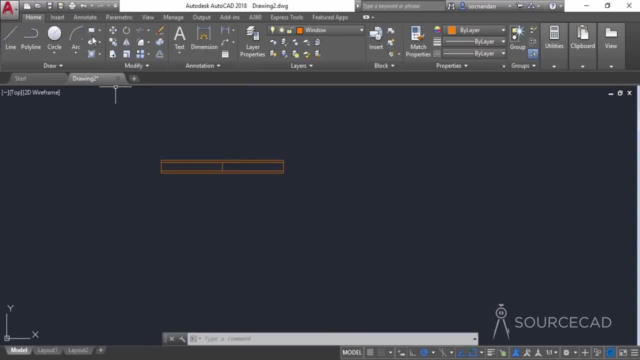 of the windows is now prepared, Let's select this rectangle tool again and make another window. For that. I'll type at six feet comma ten inches and press enter. I'll select this one, Type X, and press enter, So that will again explode, this complete geometry. 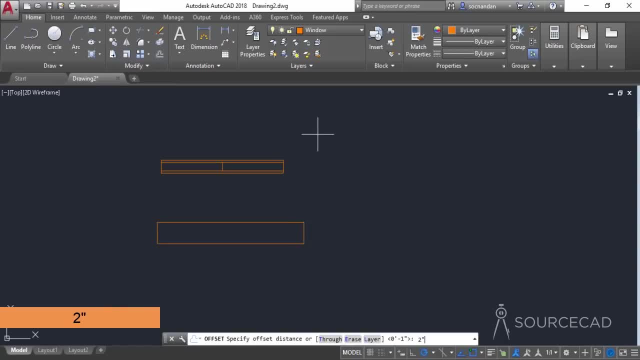 Select the offset tool Type: two inches as the offset distance, Offset this one to two inches here, Here also, and make a copy of this line, similar to the one we did in the previous case, And here also I'll trim this portion. All right, so we have these two windows and these two doors. Now let's convert them into blocks, And for that I'll go to this.